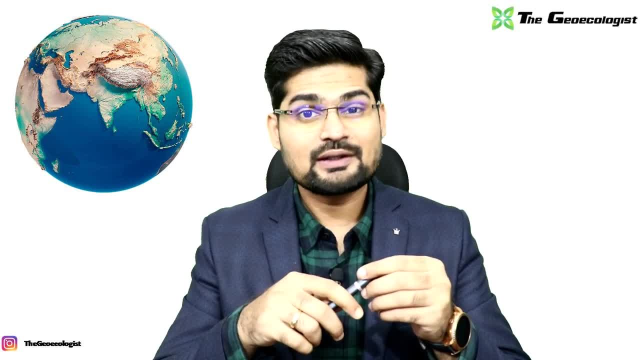 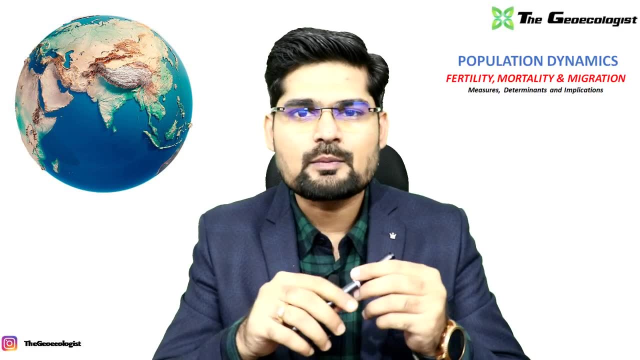 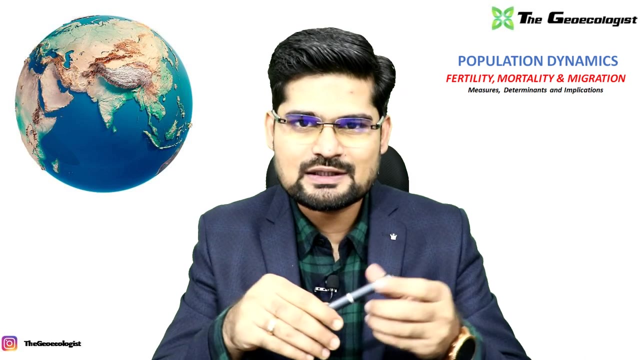 and every topic related to geography on my channel. Now, in today's session related to population geography, we are going to learn about population dynamics. Now, the concept of population dynamics involves three major pillars, that is, fertility, mortality and migration. So all these concepts and the factors and determinants related to these topics are going 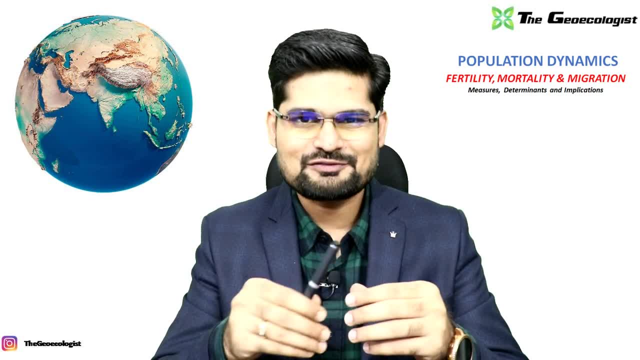 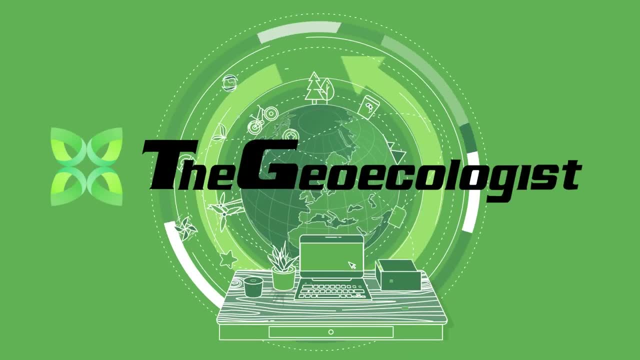 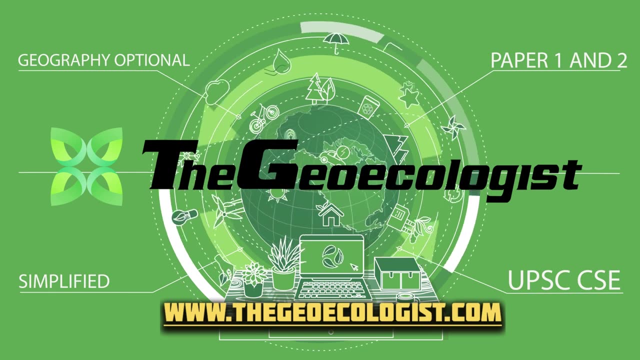 to be discussed in today's session. So, before we go ahead, don't forget to subscribe to our channel and do share the videos with others as well. So now let's discuss this topic, this concept of population dynamics. now here, the word is dynamic. now, when something is dynamic, it 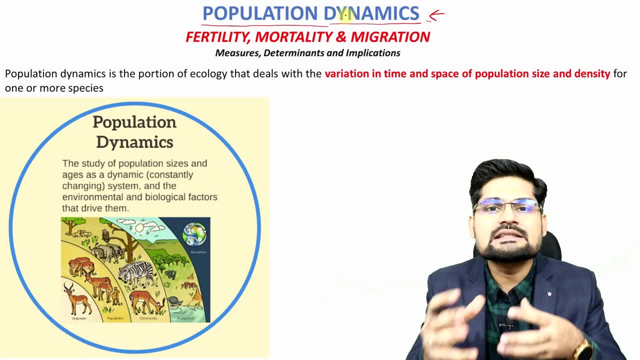 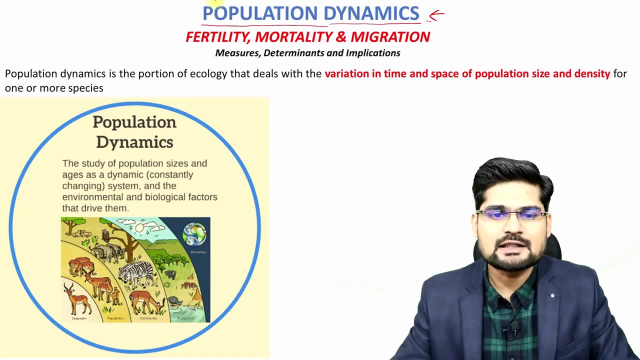 means what it's ever changing with time. there is a change in its numbers, in its spatial patterns, in percentage. that's what we look into. so here, what we are learning is the dynamics in terms of fertility, motility and migration, the three pillars of population dynamics, and also their measures. 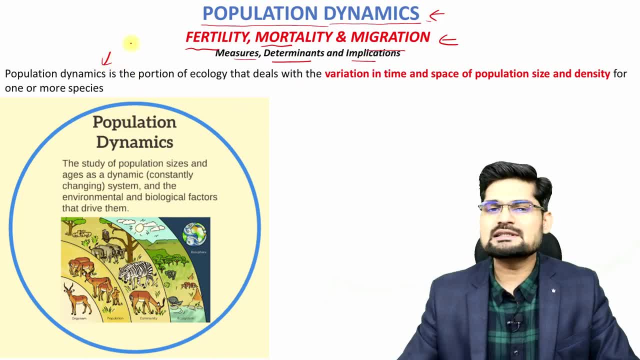 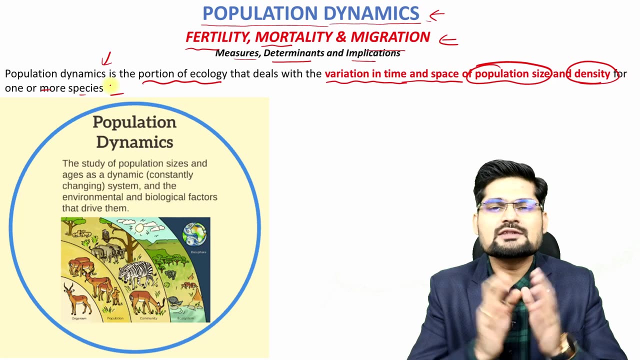 determinants and implications. so population dynamics is nothing but simply it's a portion of ecology or ecological sciences that deals with variation in time and space of population size and its density for one or more species. so in simple ways, it's not just about human population when we say population dynamics, it's basically an ecological science deals with population of. 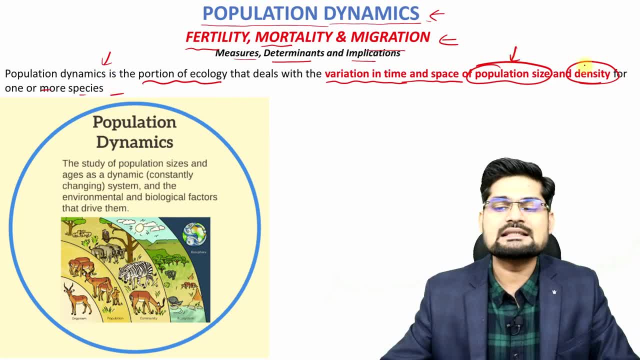 any species for that matter, where the population size and density, these two things and their spatial patterns. that's when it becomes population geography. so population dynamics is in simple ways, if you observe the population dynamics of any species, it's basically a population of any species of this diagram. what's here? study of population sizes and ages as dynamic system, right, so it's a. 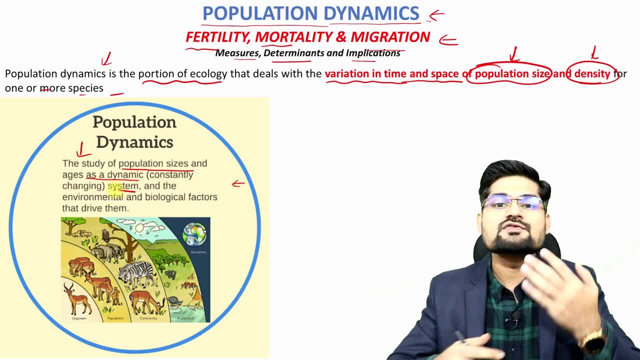 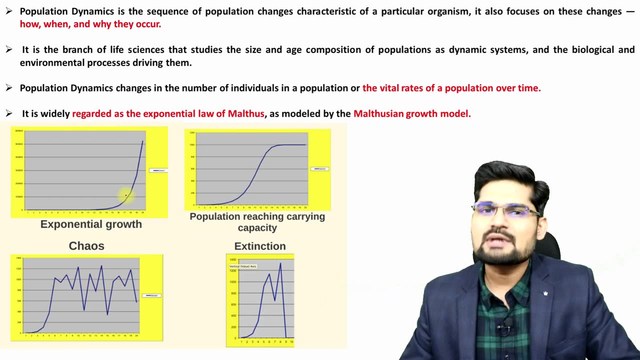 system concept. it means it will have different components which will keep changing, it will be dynamic in nature and the environmental and biological factors that are driving the system. so this is a sum, total, or a basic definition, if you can say, of population dynamics. now let's elaborate a little more on population dynamics. so it is the sequence of population changes. 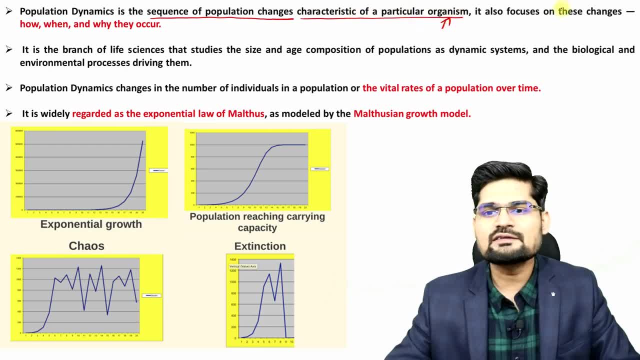 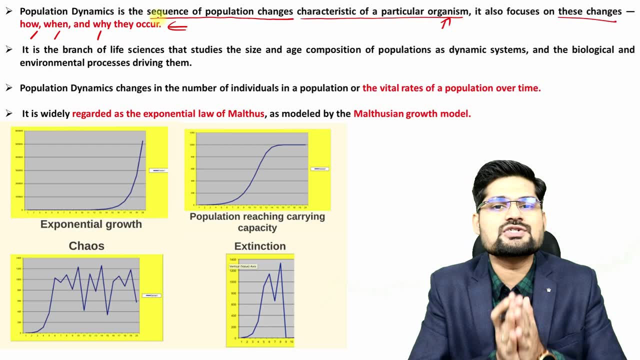 of a particular organism and also it focuses on these changes. what kind of changes so? how, when, where? why all these wh questions? if we attach to the changes of characteristics of population, that's what the population dynamics comprise of. so it is the branch of life sciences, or ecological. 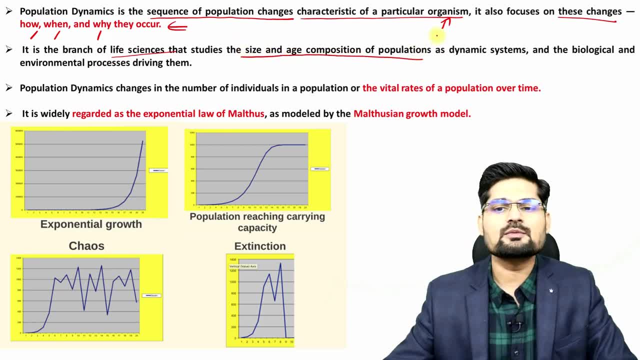 sciences that we say, where size and age composition of population as dynamic systems and biological and environmental processes driving them is studied in simple ways, or if you want to learn these kind of lines or definitions, you can use them for your and selecting as well. now, population dynamic changes, if you observe, are also the vital rates of 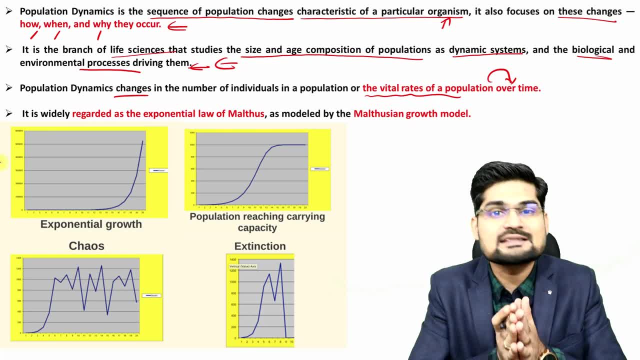 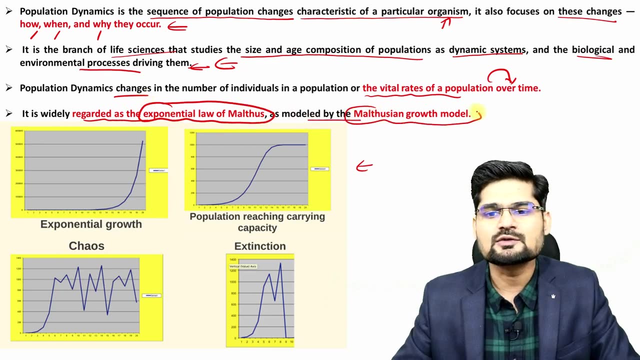 population change over time. so, if you have vital statistics of population and its changes over time- they are talking about the dynamics. now, this could be simply learned through these particular graphs, and it is also widely regarded as the exponential law of mouthers, or as modeled by the mouth, using growth model. now, if you remember, 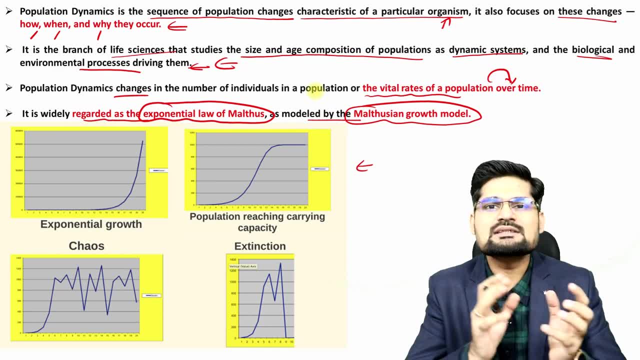 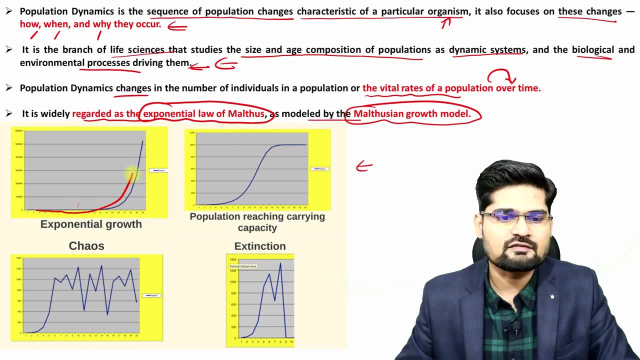 essay on principle of population by Malthus was the theory where we look into the beginnings of this kind of research. Now, exponential growth looks like this particular graph, if you observe, and then you have a particular level where at it reaches- it's the maximum carrying capacity, and also there 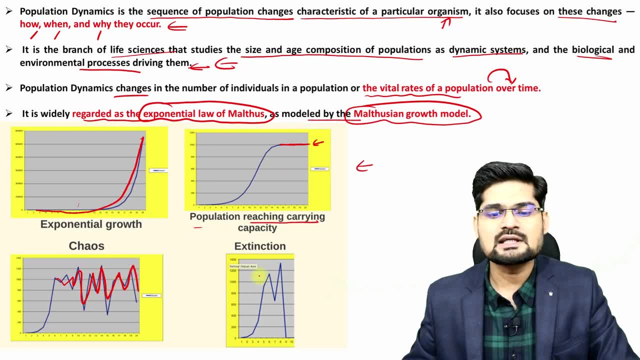 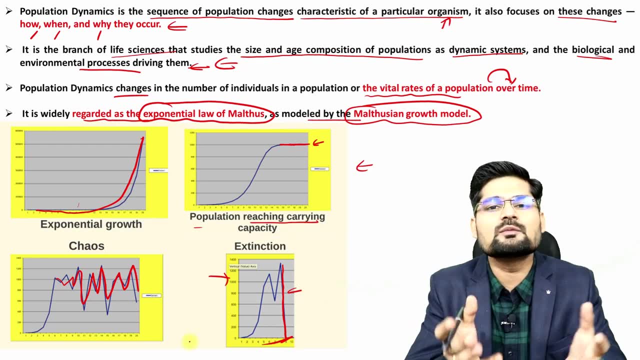 is some chaotic systems where you have dynamic fluctuations and extinction looks like this when a species gets extinct. So these are certain graphical analysis that could be potentially used, or when you are using it for your answer writing, you can use it to describe the fall rise dynamics of 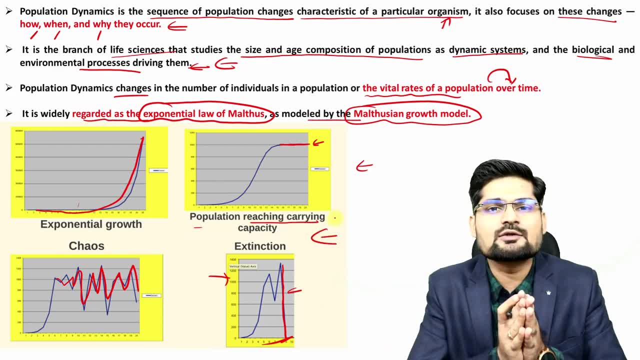 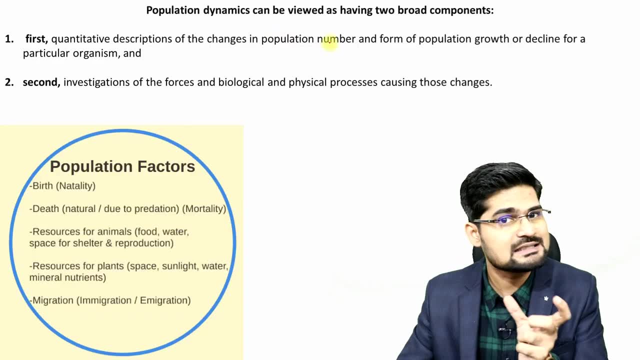 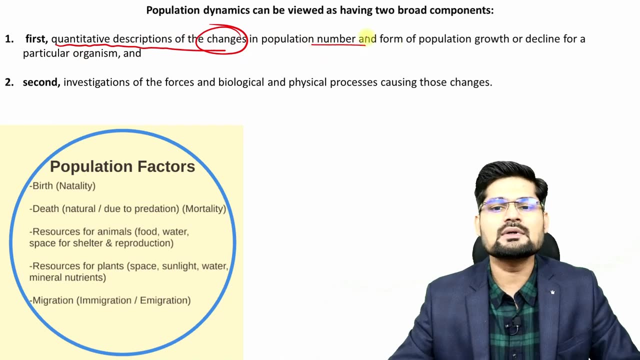 population through this graphical analysis. This is what we precisely know by the name population dynamics. now look into the population dynamics in terms of the components, because it's a system approach. So first component is the quantitative description of the changes in population, especially its number. that 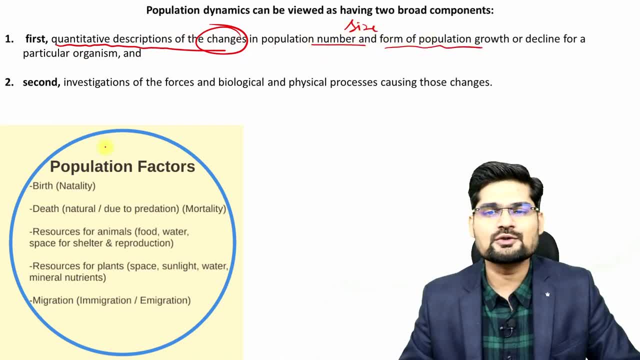 is, we say, size and form of population growth decline for a particular organism. that's the first component and the second component is the investigations, the researchers in the forces and biological as well as physical processes causing these changes. so it's not just the forms. 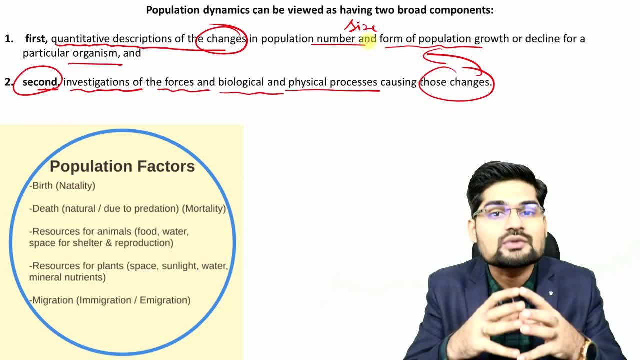 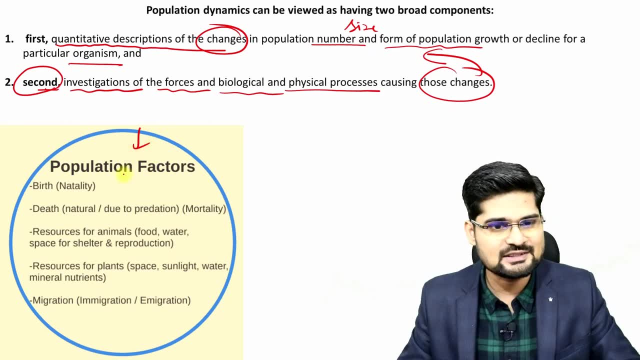 but the process, so it's process form component together. then it is the population dynamics. so look into the various factors we have also talked about in population geography in previous lectures. also the birth rate, that is, natality related deaths. that is natural or due to predation or mortality. 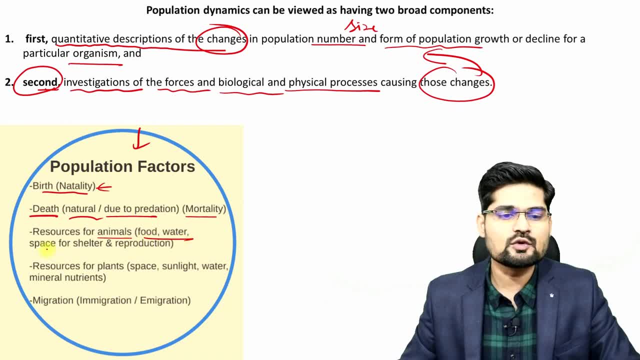 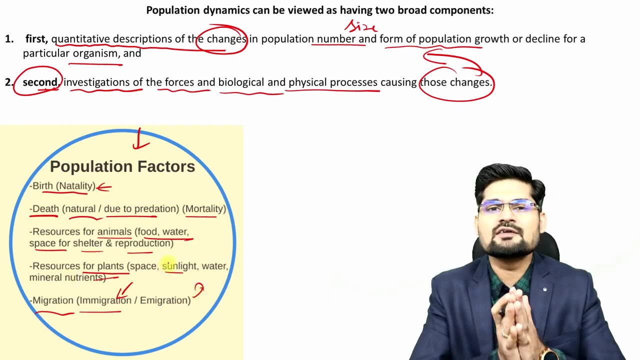 which say, then, resources for animals and food, water, space, shelter and all those things, then resource for plants as well. so space, sunlight, water, as well as the migration, the movement incoming or outgoing immigration or immigration, these are certain factors which we always consider while we are looking into these changes and the factors or the determinants talking about these. 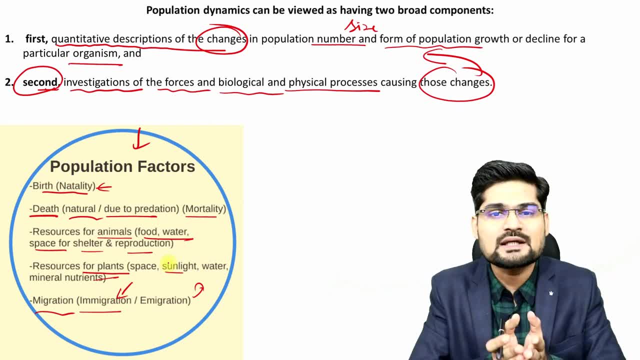 changes, making these changes in our society on a given space. so that's when it comes to population geography, when we say spatial analysis of these population dynamics, until then it's just demography. so when we look into these spatial patterns then it becomes the population dynamics in population geography per se. now look into the first. 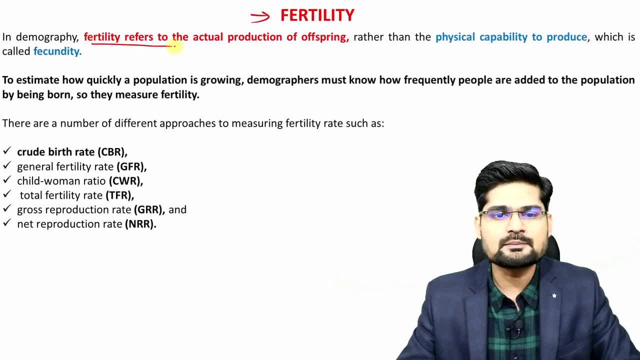 factor that we learnt is fertility. so fertility is simply the actual production of an offspring right, rather than physical capability to produce. what is physical capability to produce of an organism called? it's called fecundity right. so there is a difference between fertility- fecundity. do not get confused when you read other texts. now to estimate how quickly a population is, 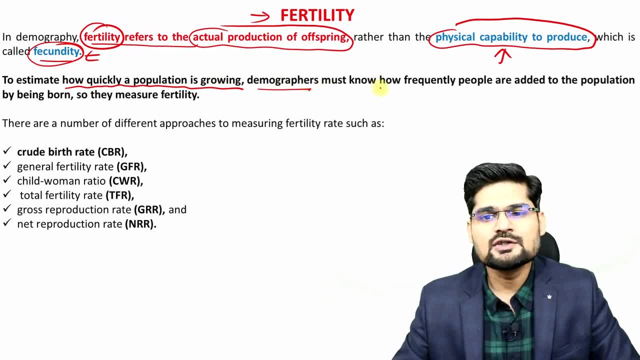 growing. demographers or population geographers also use this particularly mechanism where they measure the fertility or the birth in several different ways or different approaches. so what are the number of different approaches? look, here is the list. so it's crude. birth rate, cbr, then we have gfr, called general fertility rate, then we have child woman ratio, cwr, then total fertility. 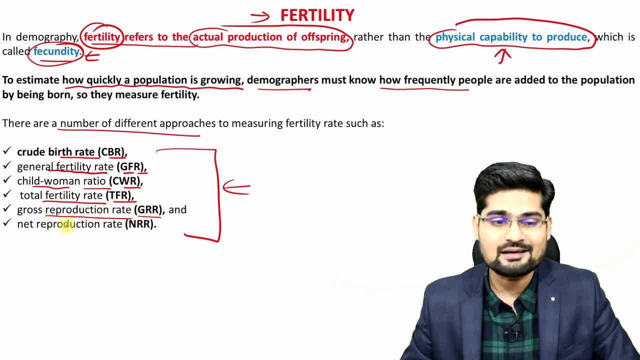 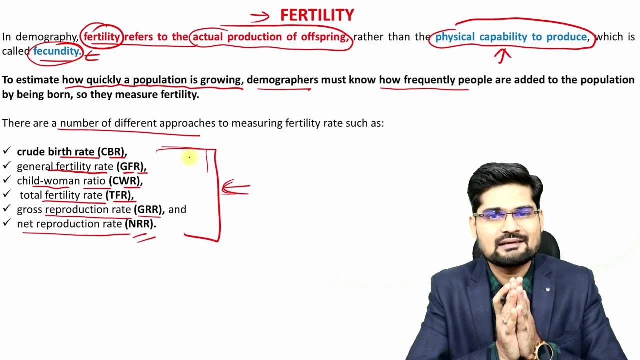 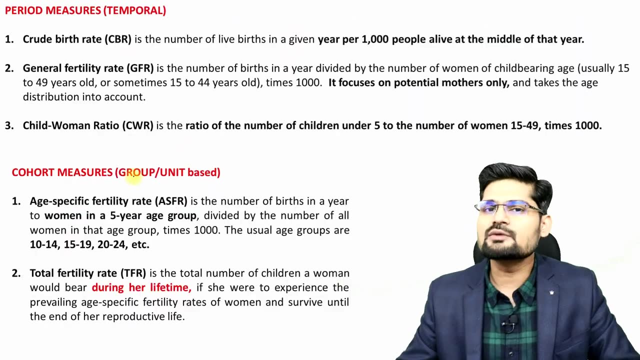 rate tfr, also gross reproduction rate grr and net reproduction rate nrr. now, if you observe, these are different approaches for measuring fertility. right, we can talk about fertility in any of these approaches when we have to use it in particular context. so, further looking at it, there are two. 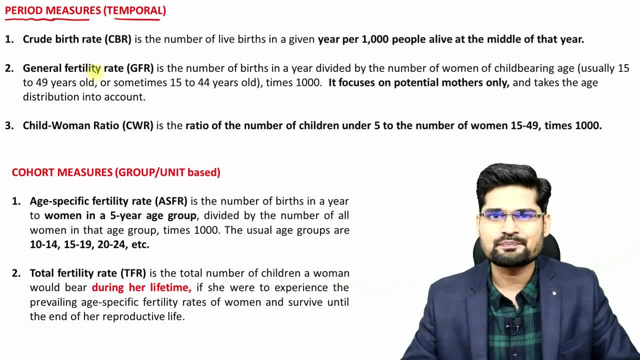 ways to measure. one is called periodic measures or temporal measures, right? so crude. birth rate is what it is: number of live births given in an year per 1000 people alive at a time. so this is the number of live births given in an year per 1000 people alive at a time. 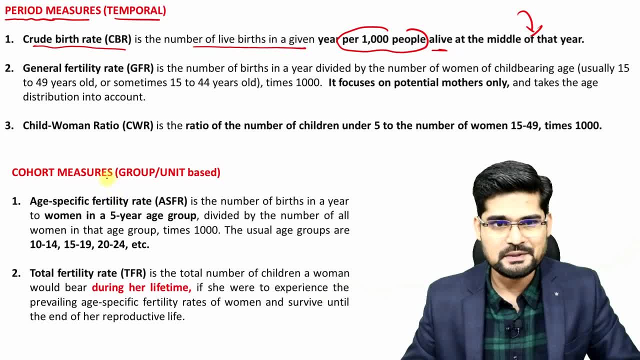 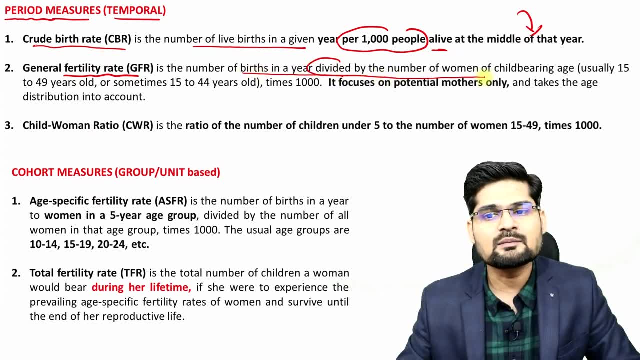 at the middle point of the year. so you see the temporal scale coming to the picture. then we have something called general fertility rate, gfr, and it is the number of births in a year divided by number of women of child bearing age. now, child bearing age is something very significant here. 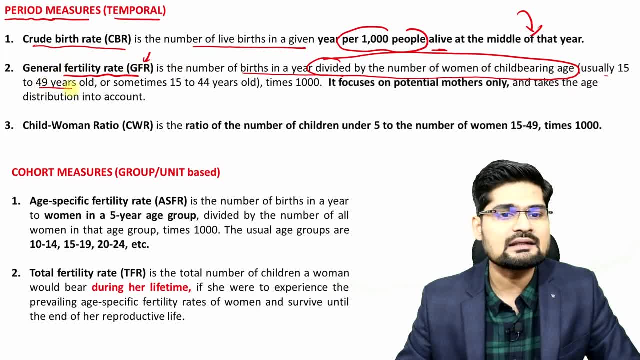 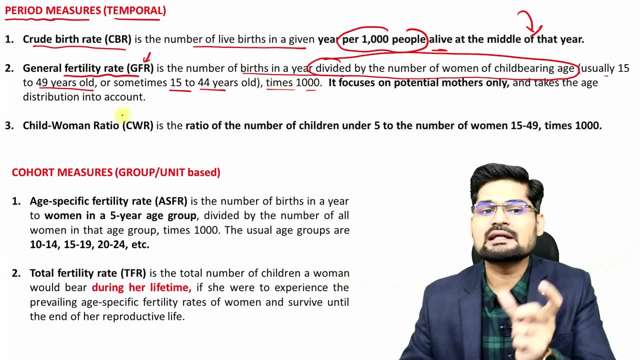 when we say gfr, because usually 15 to 49 years old is considered, or somewhere 15 to 44 also is considered, and multiplied by 1000, that's where we get that rate. so it focuses on potential mothers only now. there is a number of births given in a year per 1000 people alive at a time. so this is 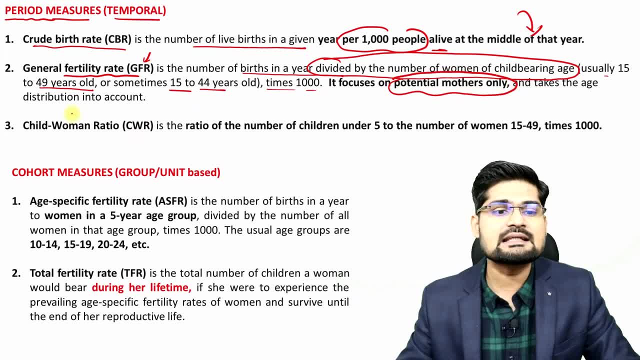 a catch here: potential mother, because it's a range and takes the age distribution into account. then child woman ratio, cwr. this is the third approach. as we learned, this is part of the periodical measures, so it's the ratio of number of children under five to the number of women, that is, between. 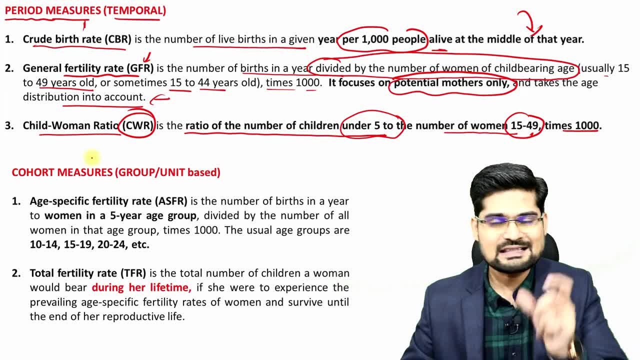 15 to 49 years of age times 1000. this rate, when we calculate, is called child woman ratio. so these are the temporal measures of periodic measures. now comes to the cohort measures, the group measures or unit measures. when we calculate the child woman ratio, we calculate the child woman ratio and we 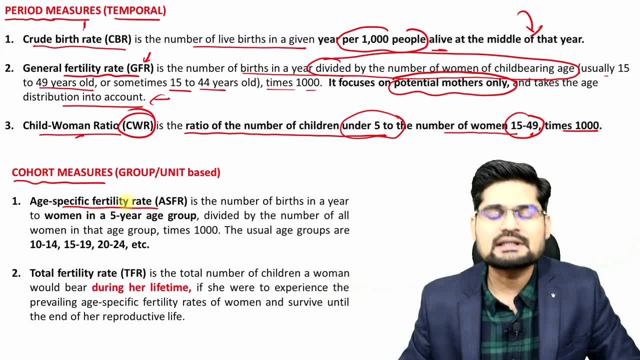 group and then calculate. so age specific fertility rate. we also say asfr is the number of births in a year to women in five year age group, divided by number of all women in that group right and into 1000. so the usual age groups that are taken here, 10 to 14, 15 to 19, 20 to 24 and so on. so this kind 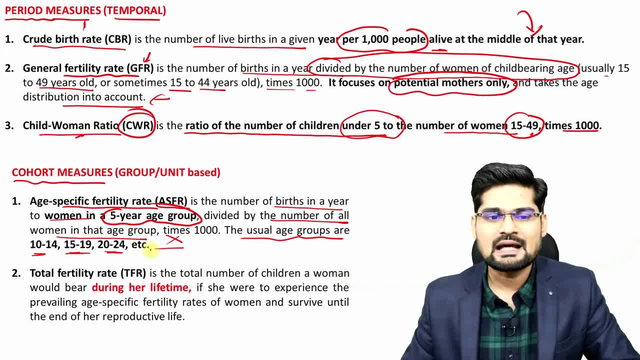 of groupings, that we do the classifications into groups and then we study. so that's age specific fertility rate. then comes tfr, which is total fertility rate, and then we study the age specific fertility rate, so the total number of children of a woman would be bearing during her lifetime. this 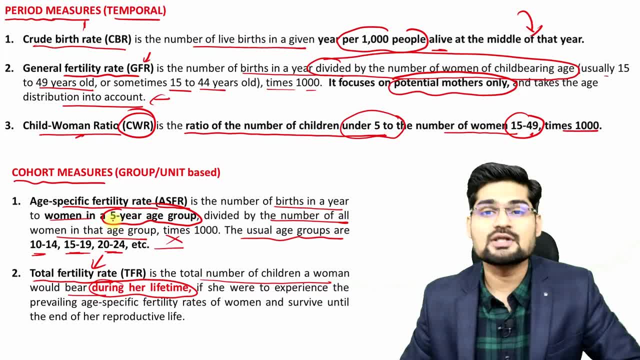 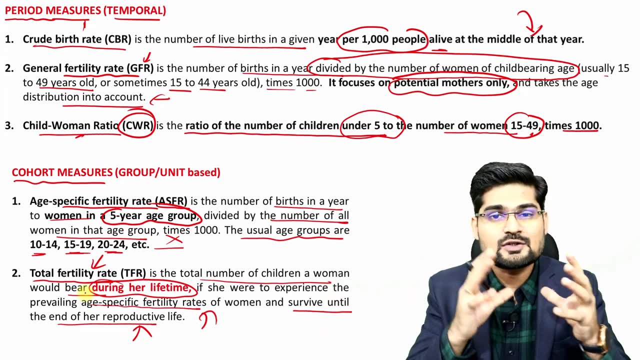 is called a total fertility rate. now, this is conditional. why? because, remember, it is age specific fertility rates that also prevails, with the same, and the survival until the end of reproductive life is also important. it means the women should survive through that entire age, right, so mortality. 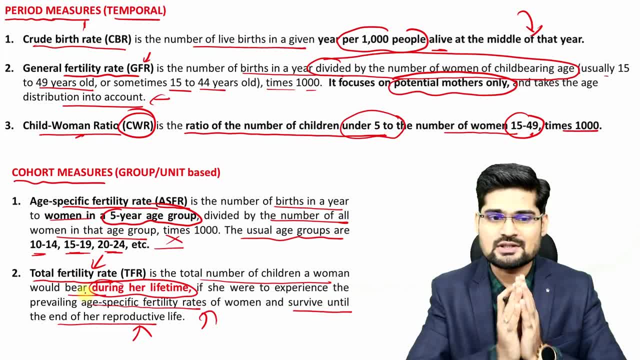 is also a picture where this kind of calculation comes into the picture. so cohort measures and periodic measures are two types of measures. so the total number of children of a woman would be ệc протester仔: lowest, longer a modul of. she lost 17 monillion missions per year and easiest. 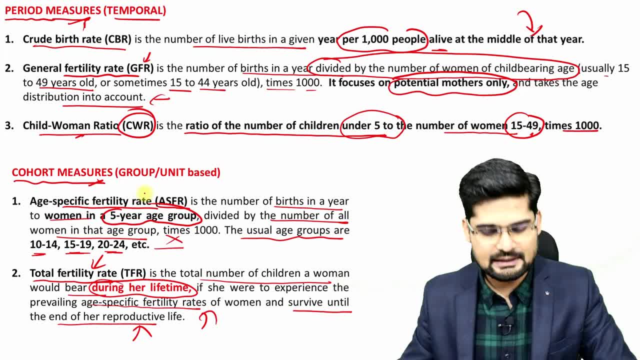 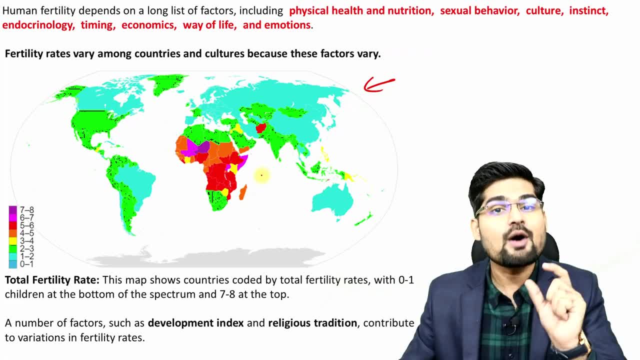 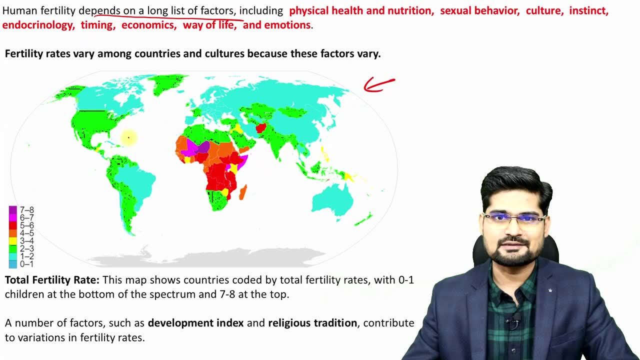 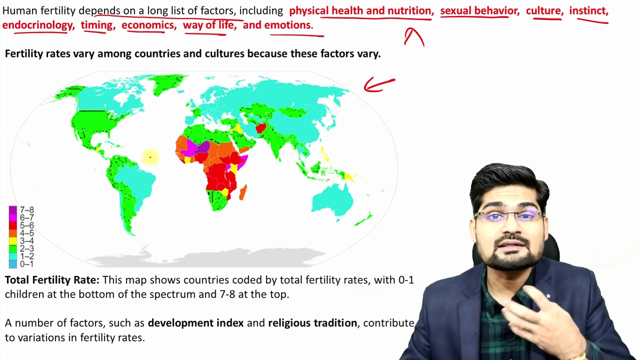 changes to weight gain, estrous weight level 26, 8 and on theふ1m, наам 25 and main. And it is a community test that 200 molecules weight and we had 160.. of life and emotions, several factors you list here. these are the factors that determine that. 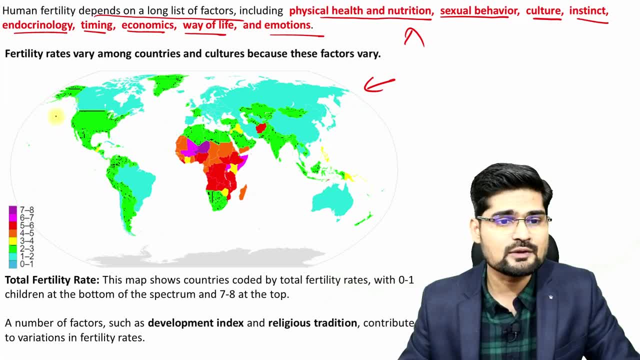 drive the population dynamics based on fertility. so if you look into the map of the world, where do you find maximum and minimum? the graph is already given here, so you observe: these areas of the world have minimum fertility. these areas of the world have minimum fertility as of now, right and the 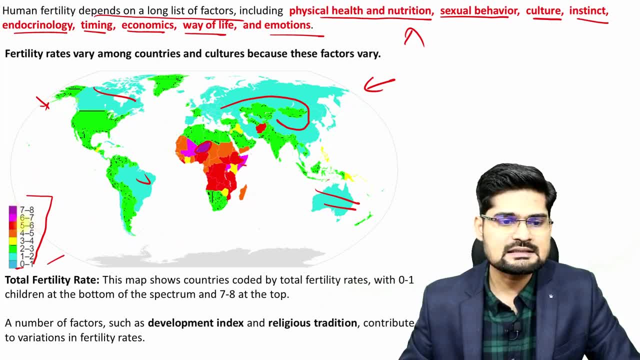 maximum is the purple patches somewhere and then these red ones, and if you observe our india, this is purely green. so two to three is the ratio here right. so we observe that number of factors of development index and also religious traditions and cultures are responsible for this kind of 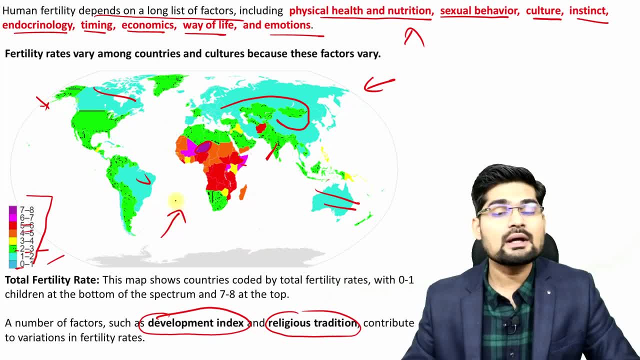 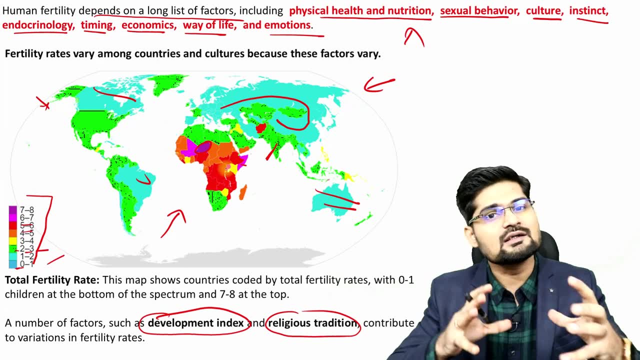 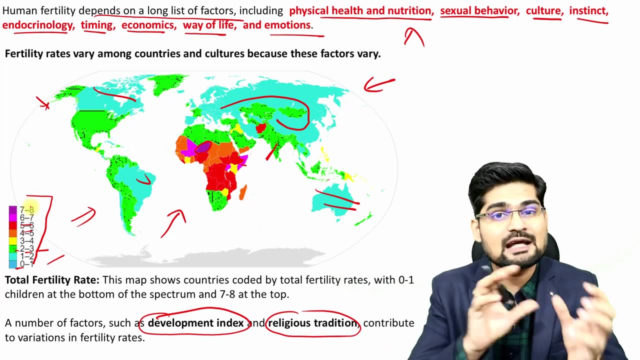 spatial pattern. so this spatial pattern reveals where is maximum fertility happening in the world and also, if you observe this map, a developed and developing divide and third world divide clearly is given out on this map using fertility rates itself. that's where we say that population dynamics and population geography goes hand in hand. 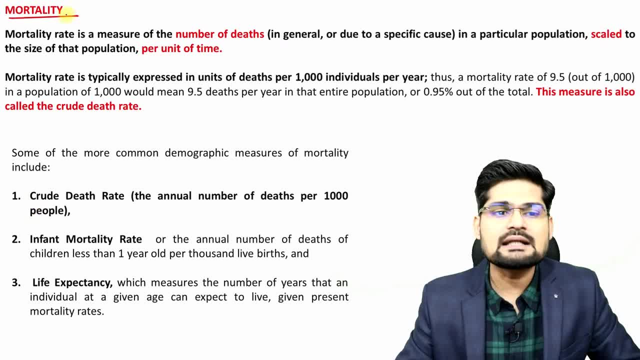 right. so now is the next one, that is mortality, now similar to fertility. we also do the mortality calculation and now here, instead of birth, we use the death. so number of deaths in general right, and causes of death could be anything right in general or due to specific cause in a particular population. 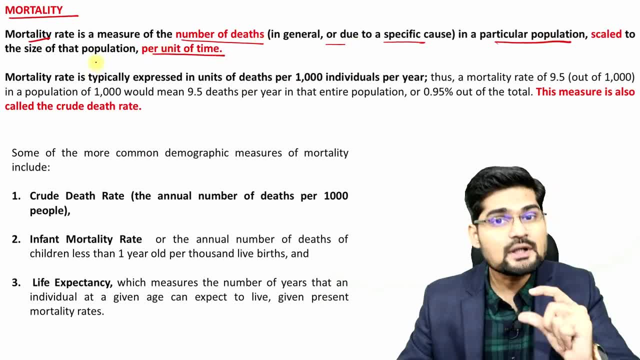 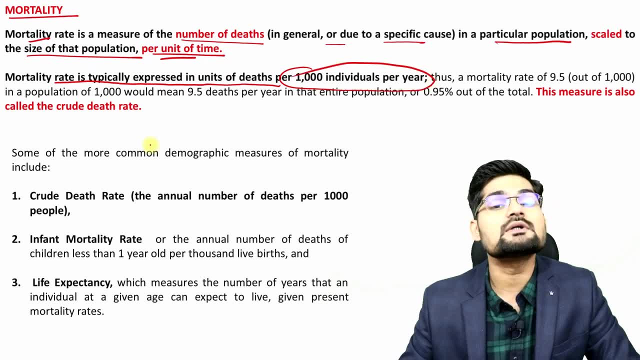 scaled according to time unit right per unit of time to be considered importantly so, mortality rate is typically expressed in units of deaths per 1000 individuals per year. for example, if you want to calculate it, suppose, say 9.5 out of 1000, so it means basically 9.5 deaths. 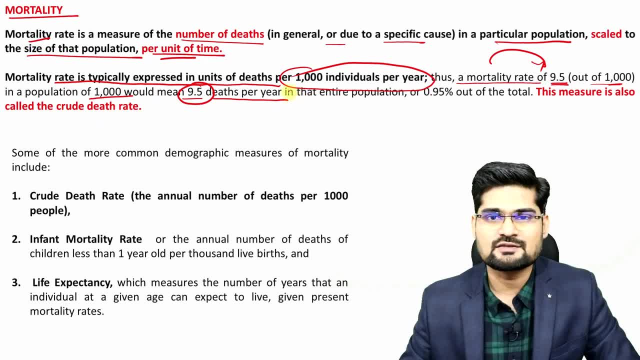 per year, per thousand of population or for the entire population. if you see right, this measure is also called the cdr, crude death rate, and there are several other measures also. so crude death rate is the annual number of deaths per thousand people. then we have infant mortality rate, very important. 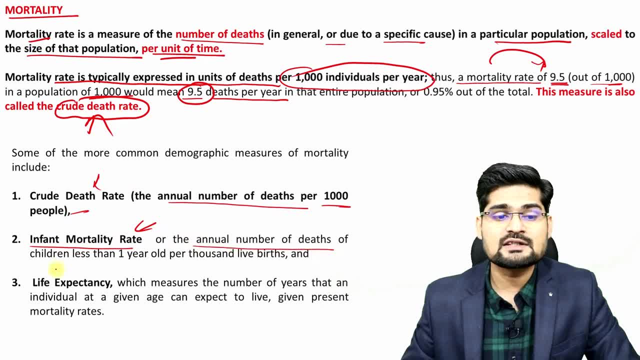 right. so infant mortality rate is the annual number of deaths of children less than one year per thousand live births. that's the annual number of deaths per thousand people. and then we have infant mortality rate. that is important, and life expectancy is also as important where we measure. 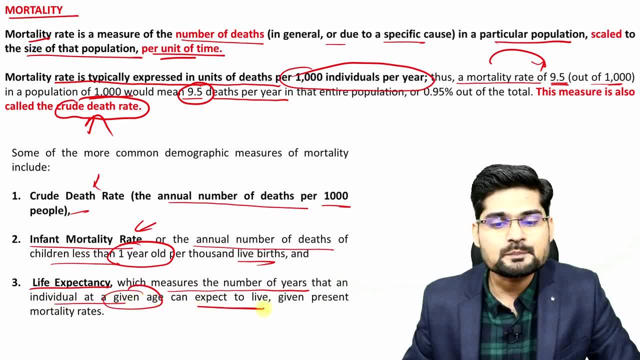 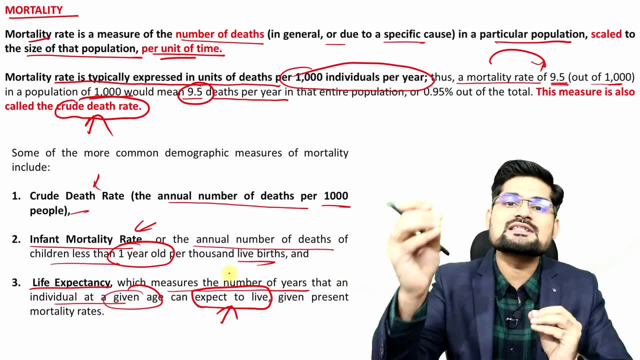 the number of years that an individual at a given age can expect to live. now, this is based on assumption that a individual given all the conditions in normal ways. so how much is the maximum expectancy of that individual now looking into the map of mortality again here, so overall, 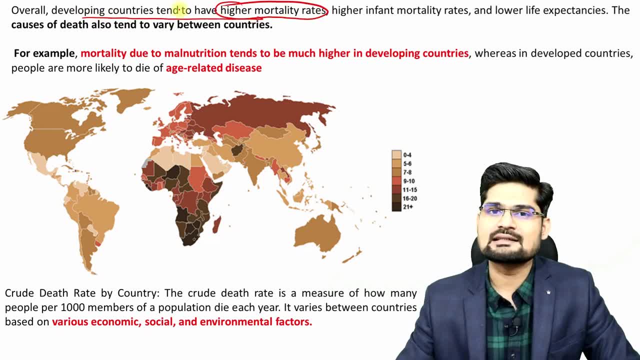 developing countries tend to have higher mortality rates and high infant mortality rates and also lower life expectancies. all the three things are observed in developing countries in these particular patterns, so the causes of death also tend to vary between the countries. that we can observe, for example, mortality rate due to. 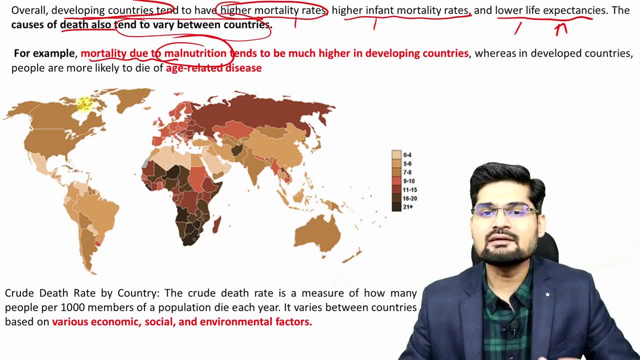 malnutrition. and where do you find malnutrition? mostly in the developing countries or far, far far underdeveloped countries where nutrition is not given. and remember sustainable development goals- we also have the food security and nutrition security as one of the important goals right so in developed countries, you will find the age-related issues. 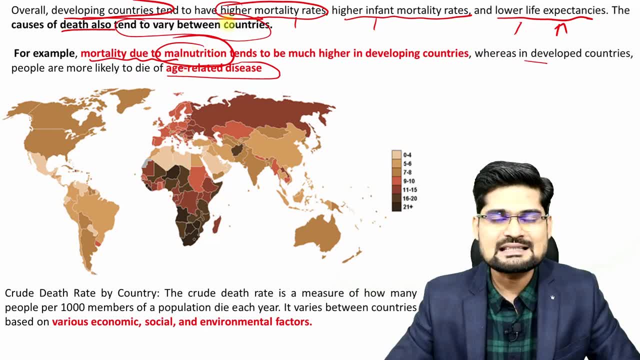 mostly in the developing countries, and in the developing countries you will find the age-related right, old aging, population or diseases right. but what happens in developing countries or third world countries that we say? that's where nutrition security and food security comes into the picture. they're far insecure, the darker ones, if you observe here. so this map gives you a picture of. 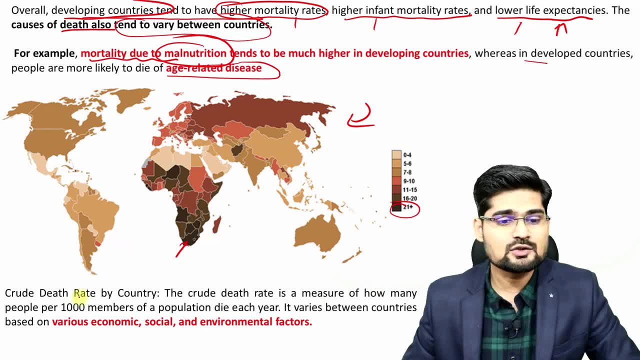 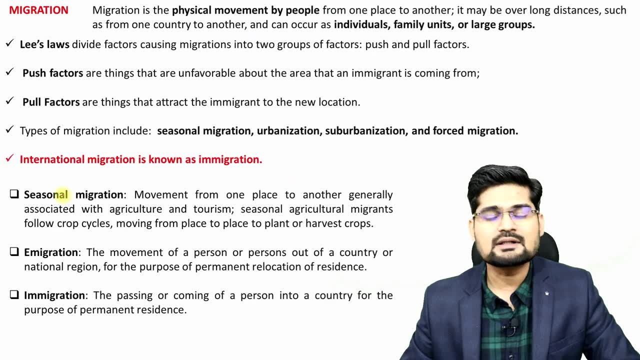 this population dynamics based on the deaths that occur. so crude death rate by country is the representation here. you can use these maps for your answer, writing now. the third pillar is the migration, so birth, death, its ratio, its dynamics. and the third pillar of dynamics is the population change in terms of migration people. 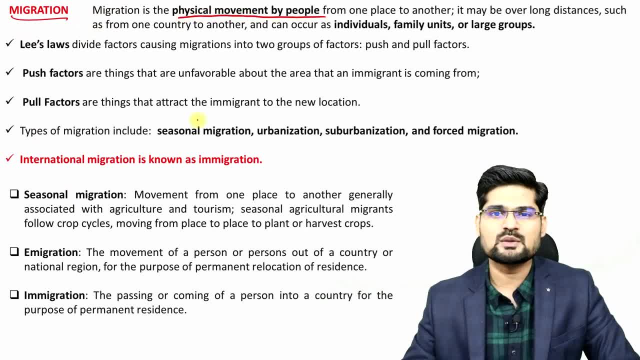 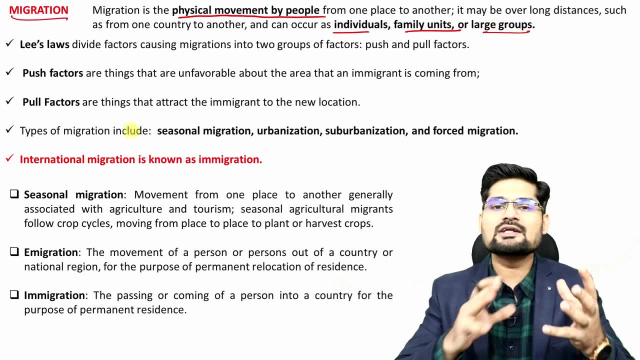 moving from one place to the other right. so this is a physical movement of people individually they move. family units also move, large groups they may moving right and since ancient times remember, migration was one of the important things. where people were hunter-gatherer, they were moving from. 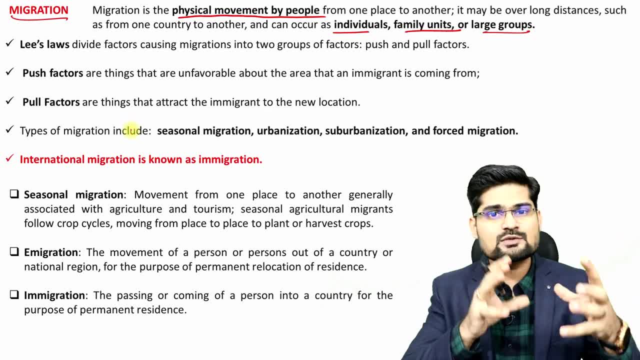 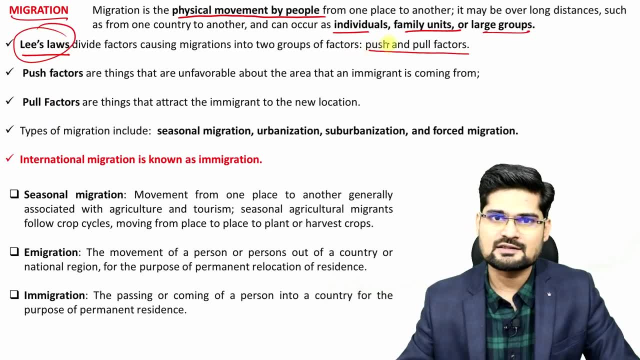 one place to the other, then start. then they started settling down. so this is where the dynamics of the pattern on the globe we observe. so lee's law, very famous- that is about push and pull factors, if you observe. so push factors are those factors which are dominant in area which pushes. 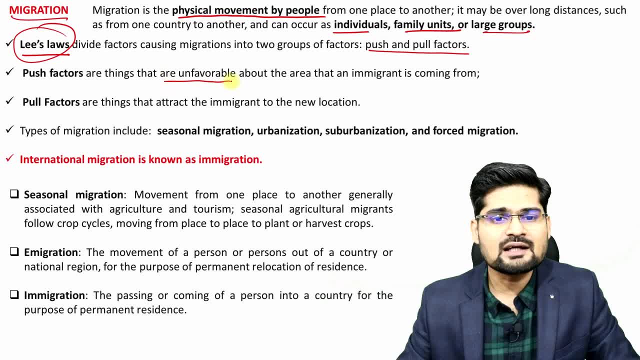 an individual to move out of that area and go somewhere else. so these are the unfavorable conditions which leads to the, which leads to the emigration from the source and immigration to the destination. that's important now. pull factors are just opposite of push factors. so when there is an 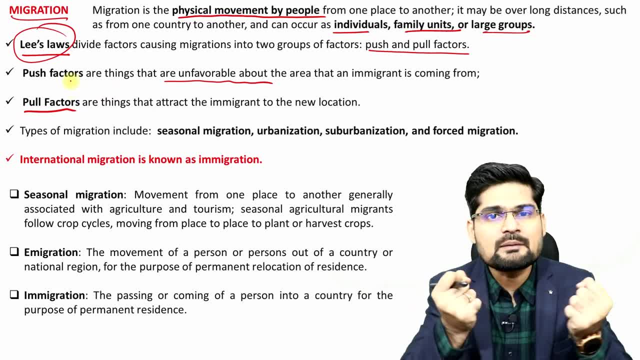 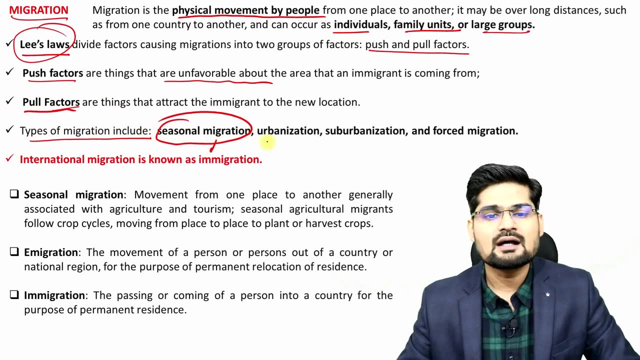 attraction at a particular place, for example, cities are pulling people because of its attractions in terms of job opportunities, health facilities and several other factors. other things right. so that's where you observe these push and pull factors and types of migration. include these major types: seasonal urbanization, suburbanization, forced migration and also now a 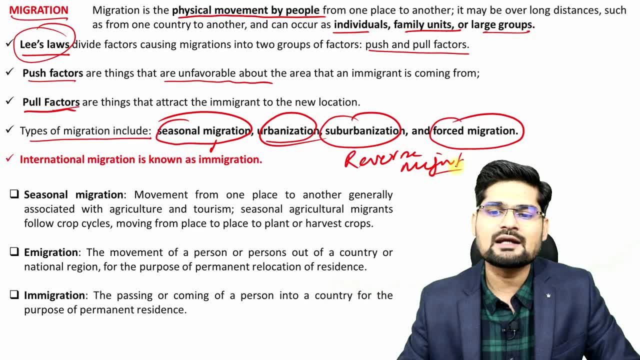 new thing is reverse migration. if you observe during pandemic people have moved from towns, cities, to the villages again, and most famous case study in india is the uttarakhand. if you have not observed it, you can check in that uttarakhand has received a lot of reverse migration during. 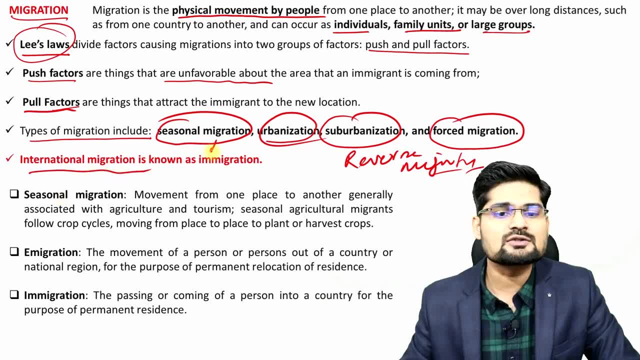 the pandemic in last two years. so national migration is also called immigration, because people are the immigrants and they have to check into the other countries where they are considered immigrants. so seasonal migration, as the word says it is. seasonal immigration is the exiting of people from one source and going out. 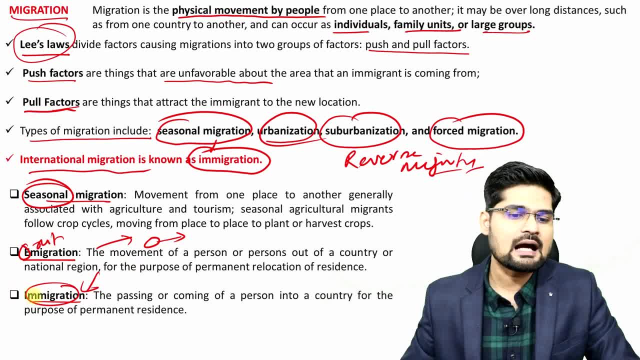 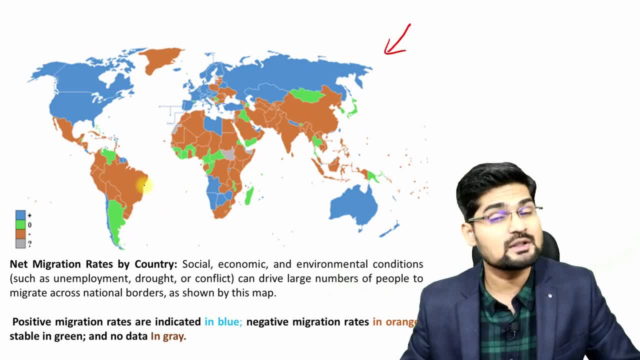 immigration is the incoming, so e is for exit, i is for incoming. that's how you can remember in simple ways. now again, let's look into the migration patterns of the world on the map. that's where it becomes population geography, right. so net migration rates by the country. if 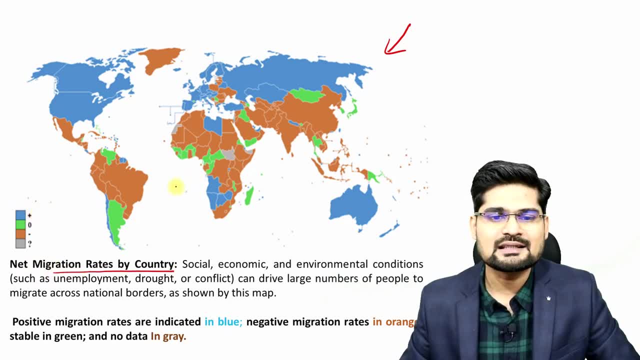 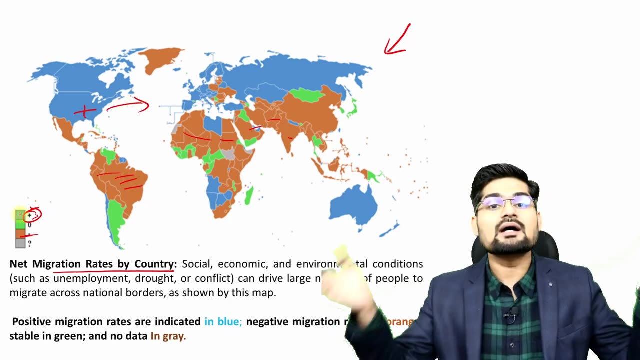 you observe which countries people are maximum migrants if you observe these brown pictures here. these are the negative ones. people flew off these countries. mostly they go out of these countries. but where you have more of blue, where you have positive ones, people are not going too much out but more people are coming in right. that's how we look into so positive migration rates are. 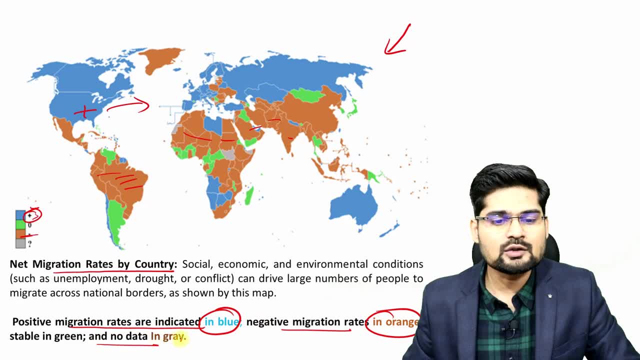 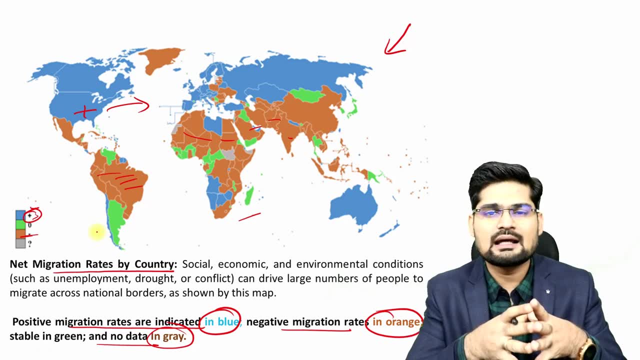 indicated in blue, negative in the orange and no data in some of the gray areas of the world that is available, right, so this is largely the language of migration when we see there is a lot of migration, of migration across the world, and now you can observe these countries and also 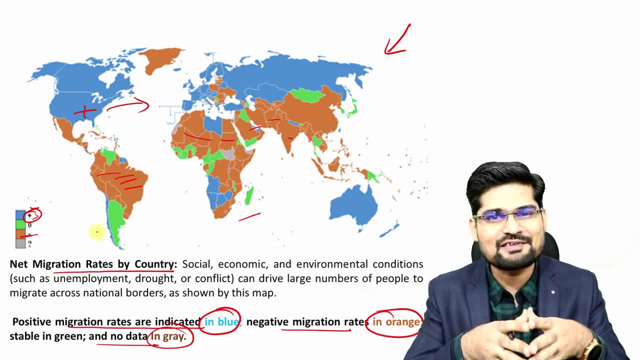 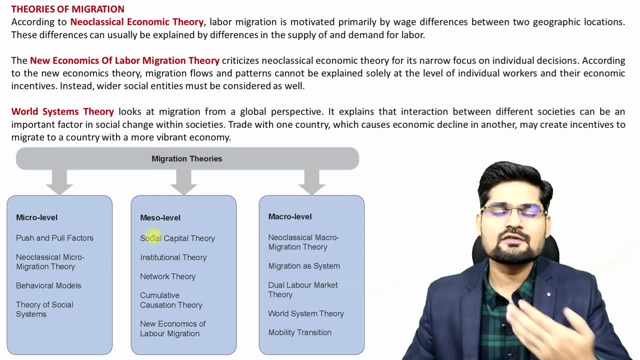 locate and clearly see for yourself how is this developing and develop divide in the migration patterns also available. so what we observe, the last point here- is the theories of migration, which talks about this support to these particular dynamics. so what are these theories? neoclassical economic theory which says: 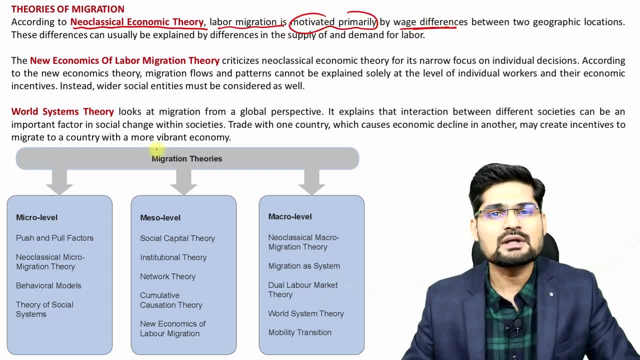 labor migration is motivated by wage differences. primarily, economics determine the migration. that's what the neoclassical economic theories, then neo-economics of labor migration theory, criticizes these neoclassical theory and says that it has a narrow focus only on individual decisions. so, according to, 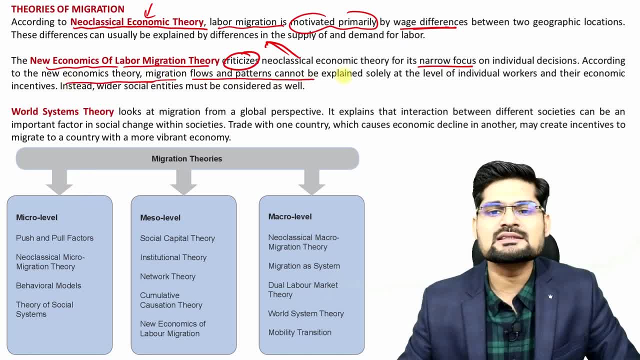 this new economics theory. migration flows and patterns cannot be explained solely on individual workers and their economic incentives. instead, we also need to look into the wider social entities and the processes that operate in multitude. that's what the thing is. and then there is something called world systems theory. so world system theory: talk about a system concept where it's a. 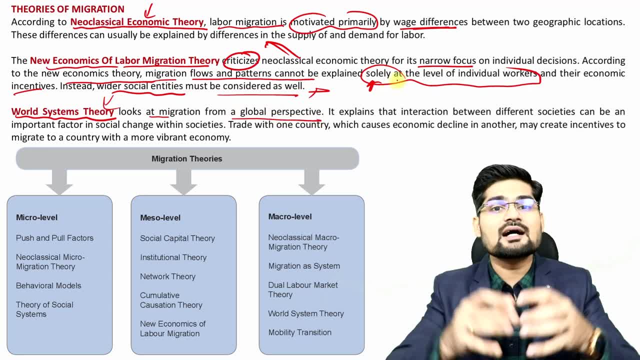 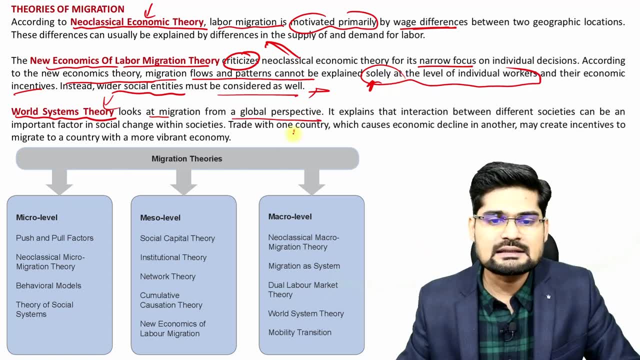 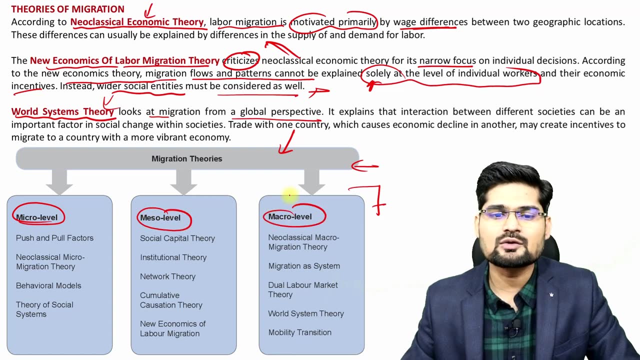 global perspective where different kinds of factors, agglomeration of factors, right that is taken into consideration, which drives the migration of people. so, in simple ways, this could be one area where you could practice this kind of flow diagram for yourself at different scales, so micro, mezzo and macro. what are the theories? 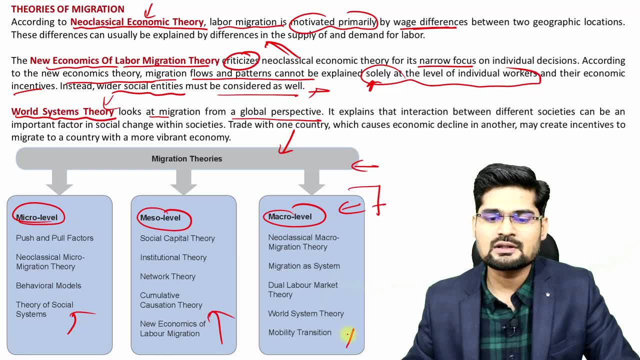 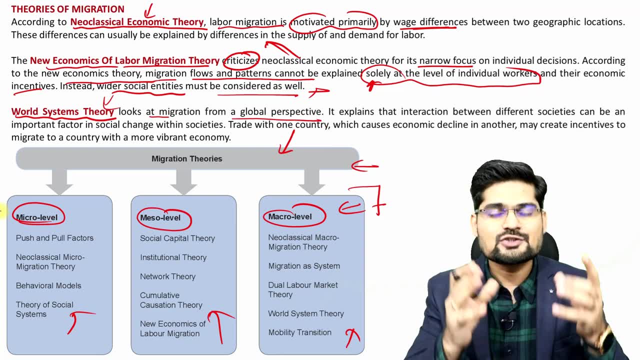 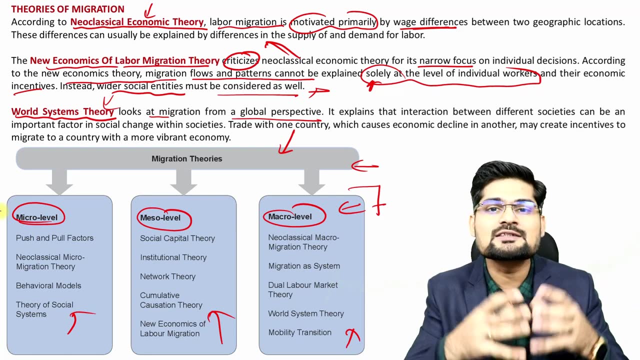 that are involved and here is the list of the theories. you can pause the video here and note it down and in details will be talking about more migration related concepts in the lectures to come separately. so here in this lecture we We talked about majorly the fertility, mortality and migration and its spatial patterns, global patterns and its dynamics across the world. 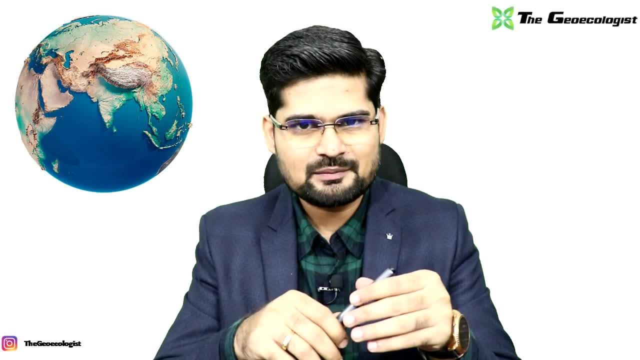 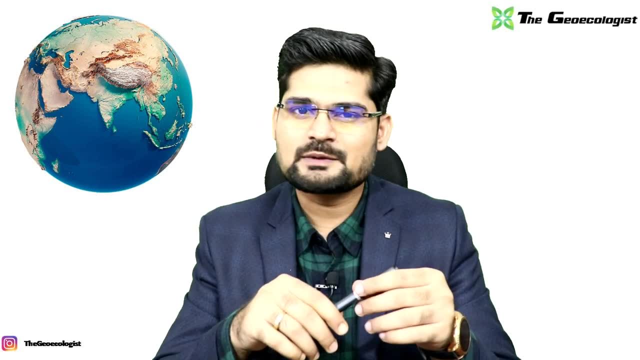 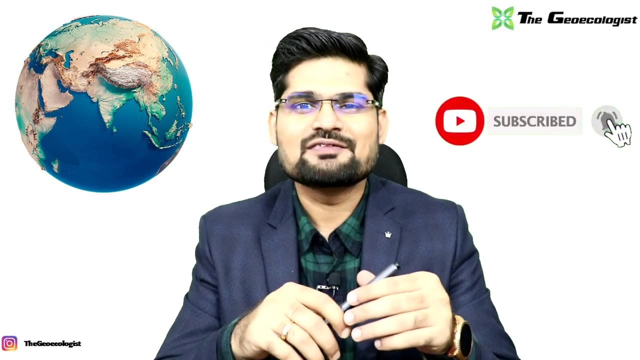 So now when we have learned in details about the population dynamics- various factors, attributes, examples through the world- in the sessions to come we'll be talking more on different other aspects of population geography. So stay tuned, keep watching and learning, and don't forget to subscribe and share the videos with others as well. Subtitles by the Amaraorg community.